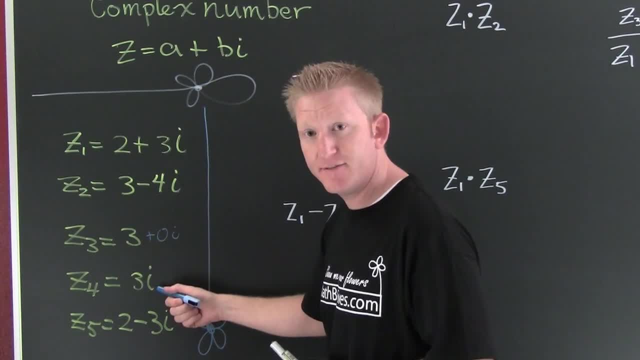 of complex number, It's purely real. Down here I have z4.. That's purely imaginary. It doesn't have a real part, It only has an imaginary part. And then I have this last one down here for you: z5.. This is 2 minus 3i. Let's go through some of 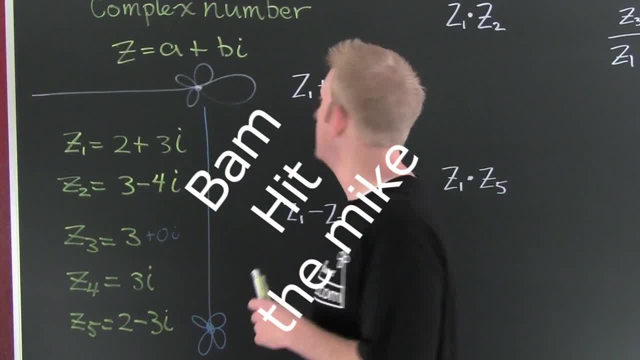 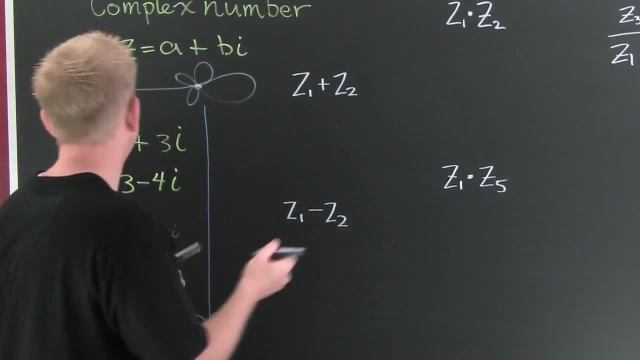 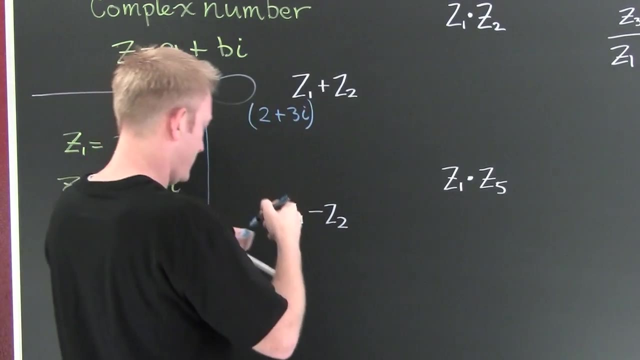 these operations with complex numbers. Okay, sure, First, what I want to do is I want to add z1 and z2.. I'll put those up here for you. This is um 2 plus 3i And I'm going to take that and I'm 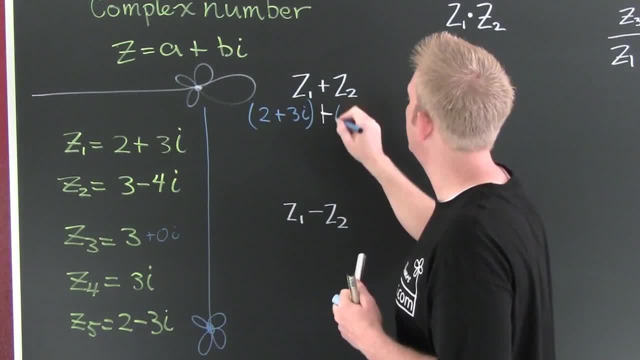 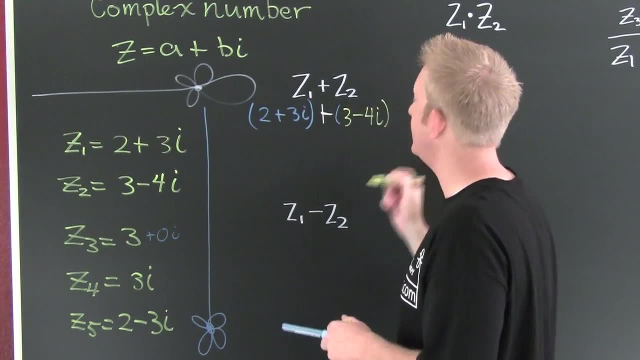 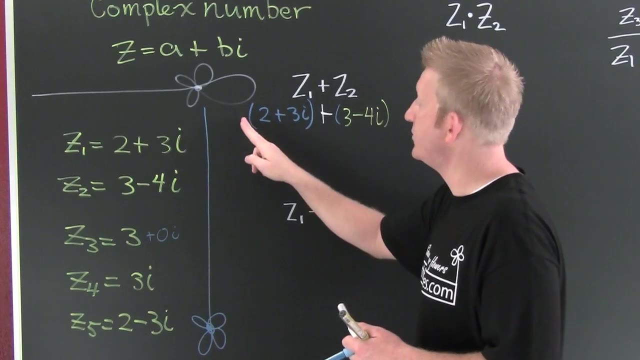 going to add it. to Put that in yellow: 3 minus 4i, I'm adding z1 and z2.. So this is how you add z1 and z2.. These parentheses are unnecessary. There's no number in front and no minus sign in front. So then we're. 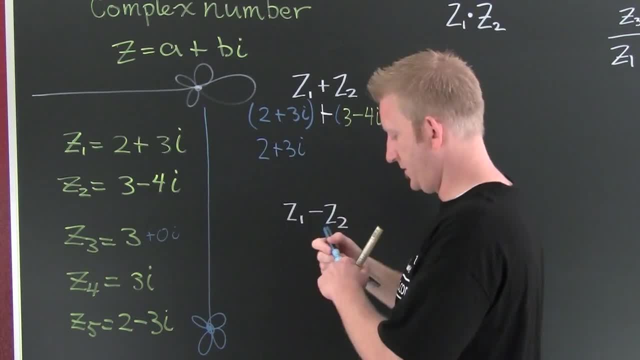 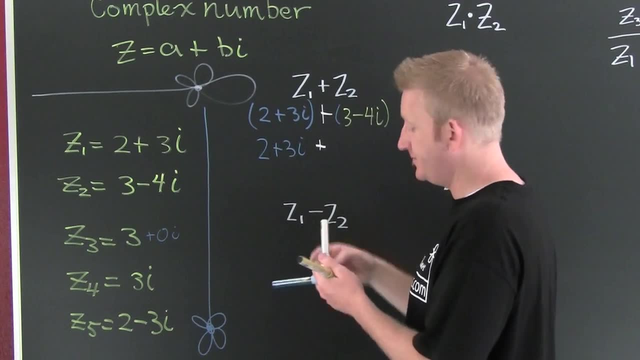 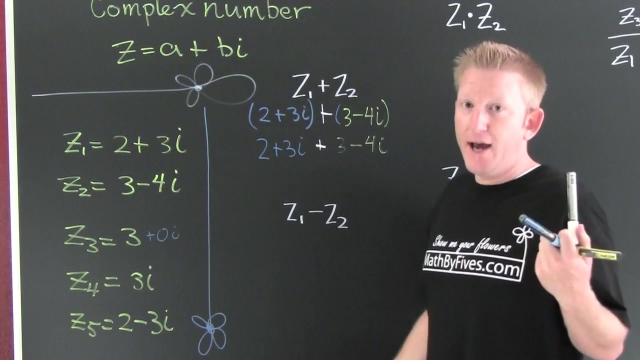 going to have 2 plus 3i plus. These parentheses are unnecessary. No number in front, no minus sign in front. 3 minus 4i. Okay. So now when we're adding these, Adding and subtracting these complex? 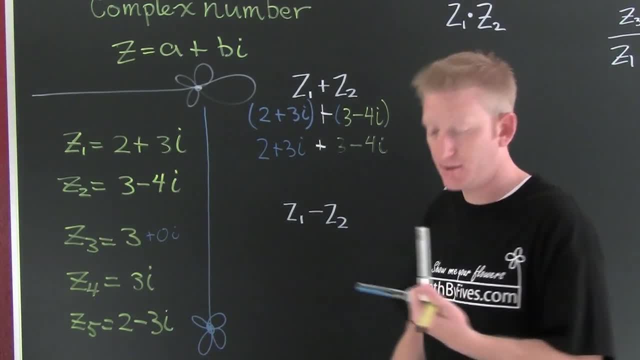 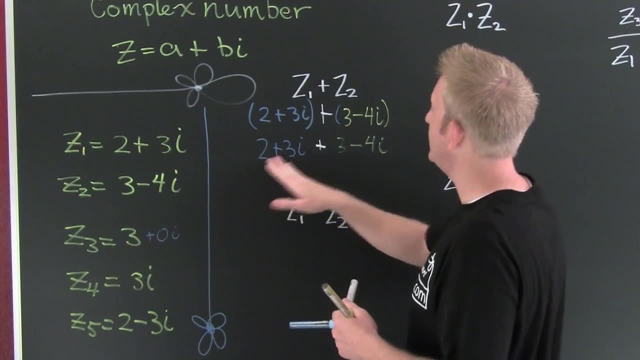 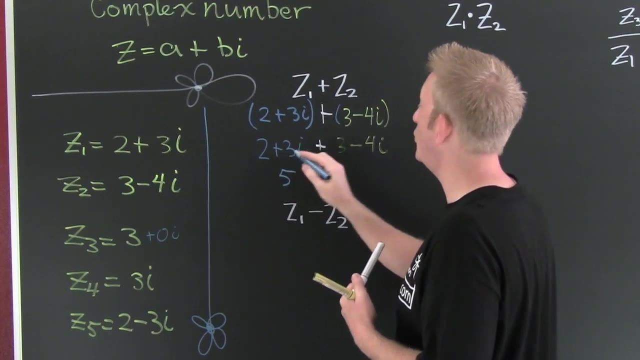 numbers. we add the real parts and we add the imaginary parts. It kind of feels like gathering like terms, but it's more like gathering like places. I have 2 reals and 3 reals Together it's going to give me 5 reals. Yes, Ooh, 3i minus 4i is going to give me a minus i, I-i-u. 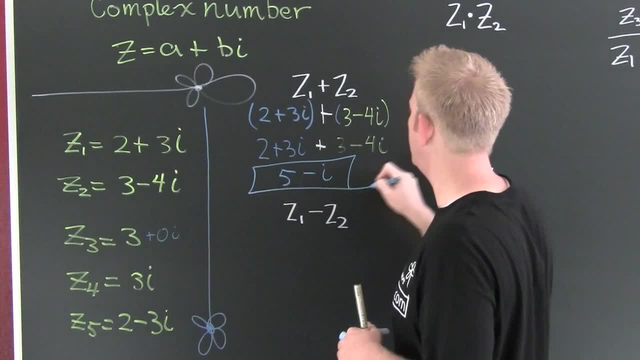 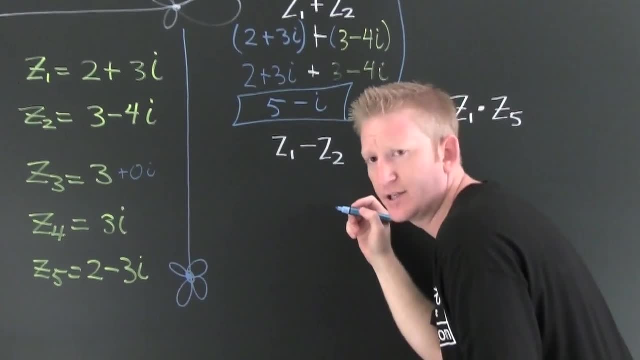 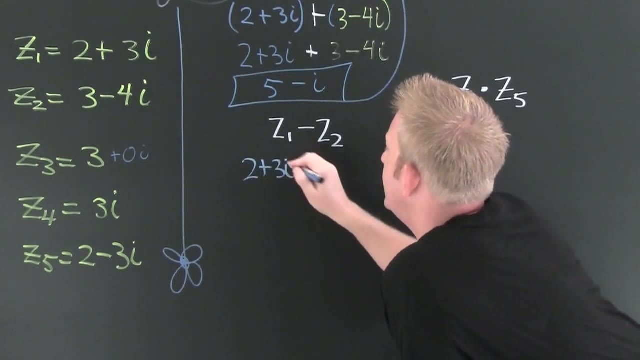 I-i-u And a flower. Down to subtraction. Okay, Here I'm going to take z1,, which is going to be 2 plus 3i, And I'm going to subtract off this time Z2,, which was 3 minus 4i. Okay, 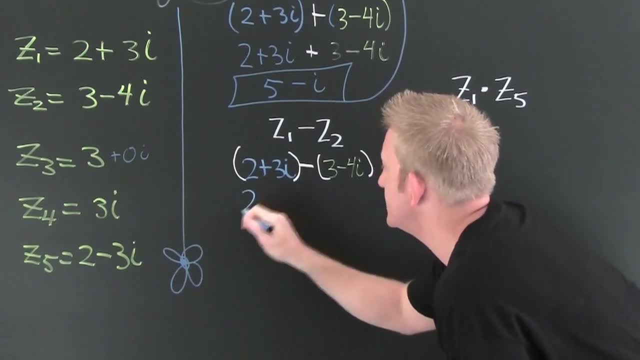 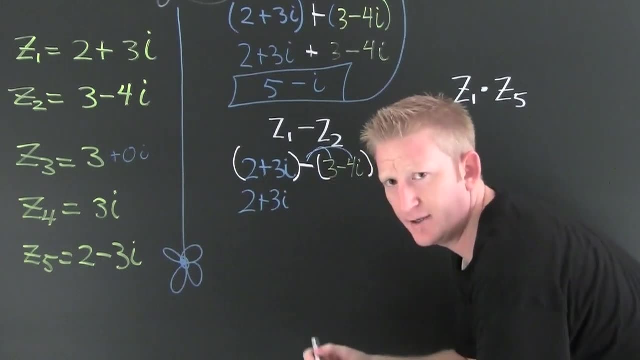 So here these parentheses are unnecessary. This is 2 plus 3i. These are necessary. Oooo-t, Oooo-t. Because it had the minus sign on the outside. You can change the sign. I have everything on the inside. It becomes a minus 3 and a plus 4i. Okay, Gather, collect and combine. 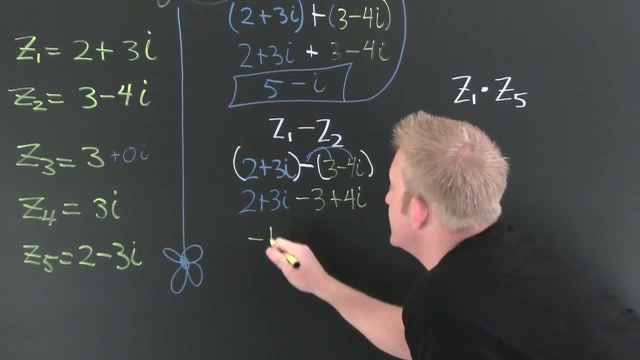 Well, they're not really. Yeah, okay, Real part. real part, That's a minus 1.. Fun, Imaginary, imaginary Plus 7i, And at that point we typically write the i out back, because that's how our complex. 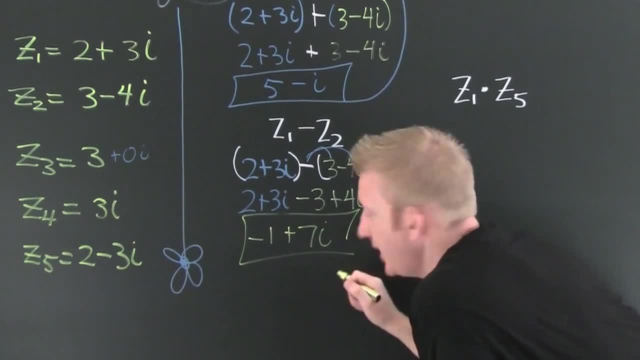 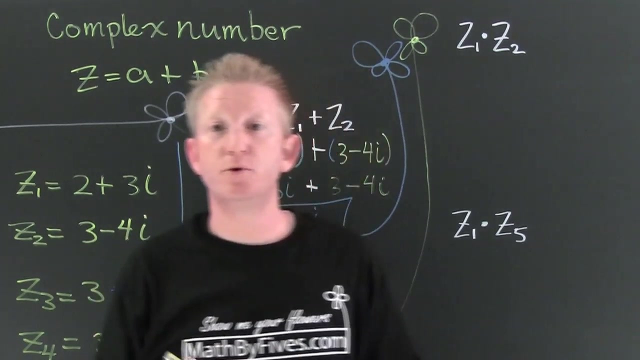 numbers are written Real plus imaginary, Okay, And the ii-ii-i-ii-i i unit signifies the imaginary part And a flower. Okay, Let's talk about how to multiply these things. Let's look at a little z1 on z2.. 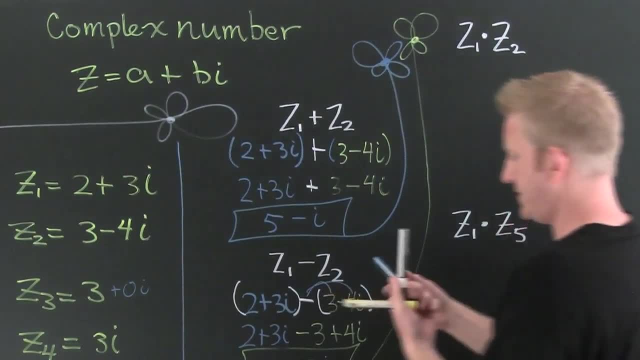 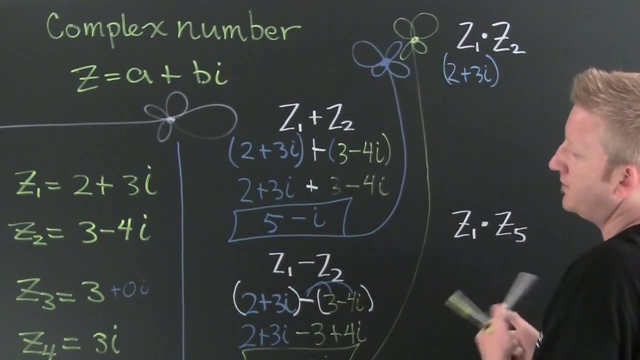 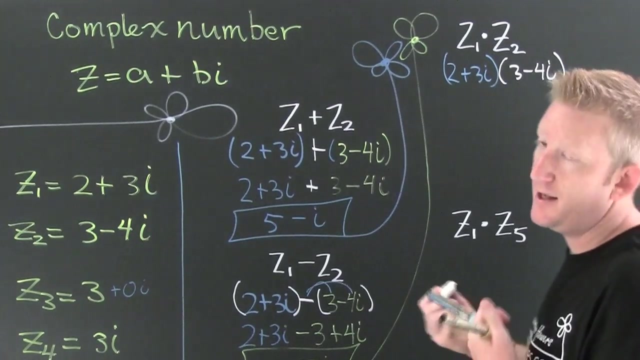 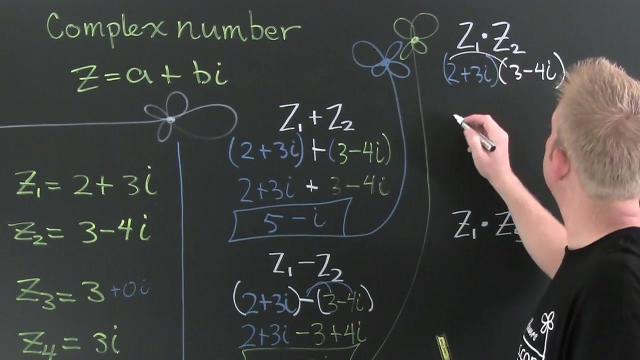 one Aussie to action, mm-hmm, yes, so then I'm gonna take two plus three, I, and I'm gonna multiply it by three minus four. okay, so then I have two turns on two turns. I'm gonna first in or out of last it. yeah, okay, this one times that one. 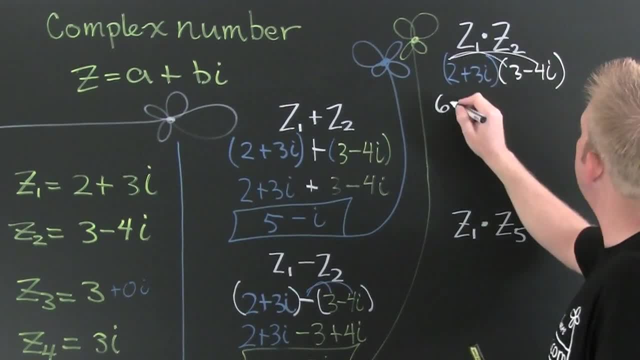 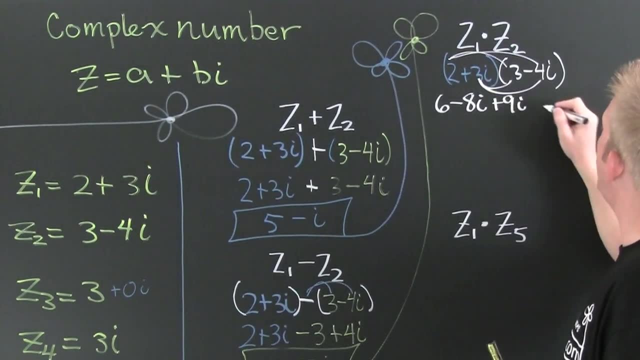 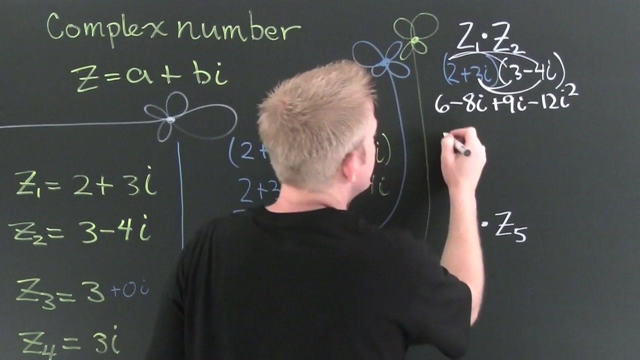 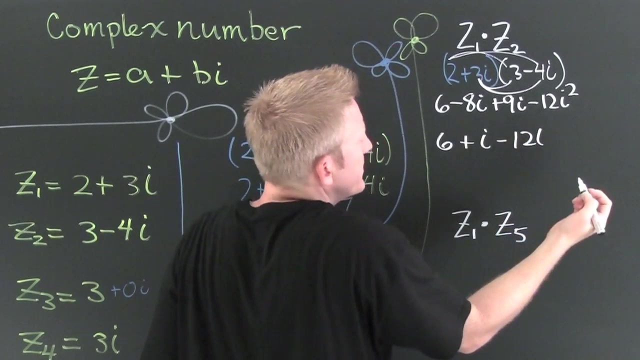 that's six. first outer is minus eight, I inner that's plus nine. I last minus 12 eyes squared. now we gotta clean it up a little bit. this is six, boom plus. I wait for it- minus 12 times. what was I squared from a previous video? yeah, minus one, fun. 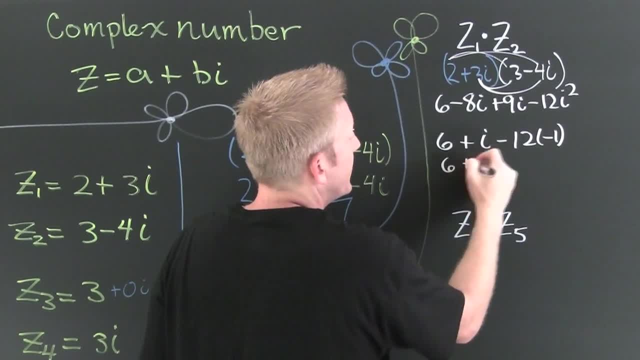 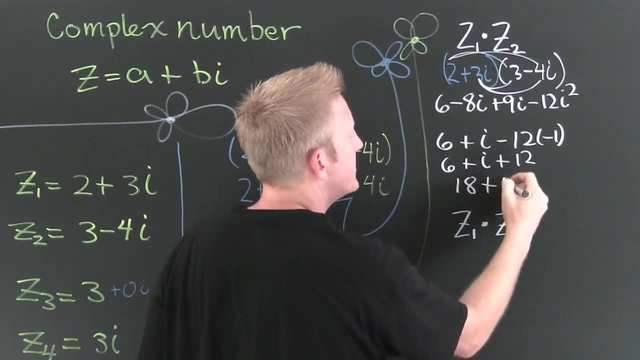 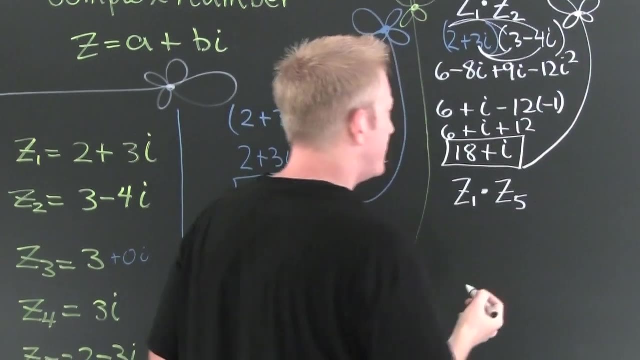 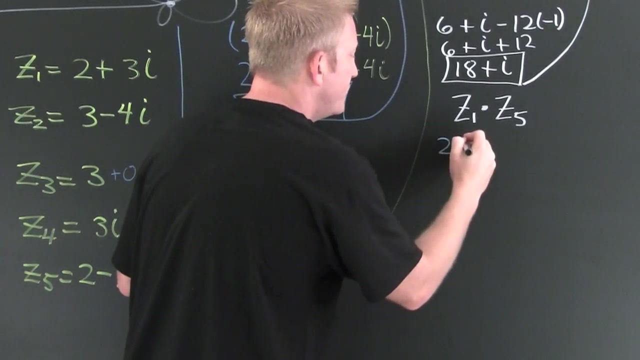 oh yeah, you like that. so then this is six plus I plus 12. 6 and 12 gonna get you 18 plus I. okay, let's take another product, hmm, kind of special here. I'm gonna take two plus three I and then multiply it by two minus. 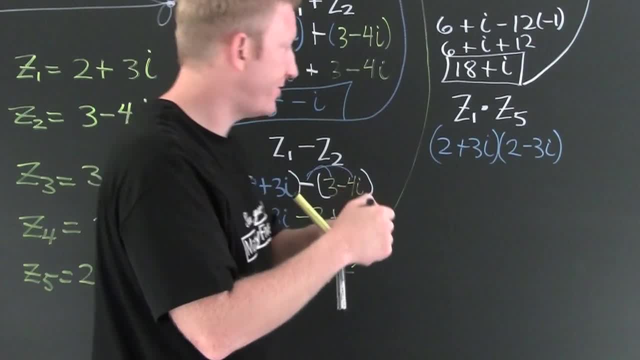 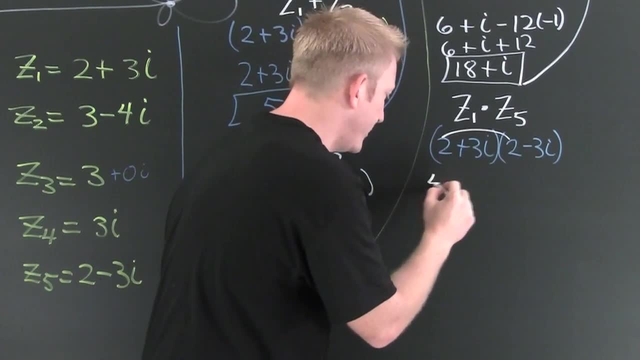 three I. that's your z-1 and your z-5. ح sine. I'm gonna first in, or power lasted. this is um 2, 4, sure. the outer is minus six. Einstein said Z1, z-11 second instead of Green in first, inner, add in last it. this is um 2 for sure. the outer is minus 6, I the. 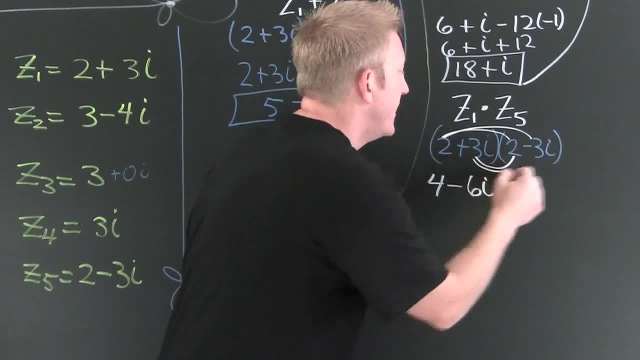 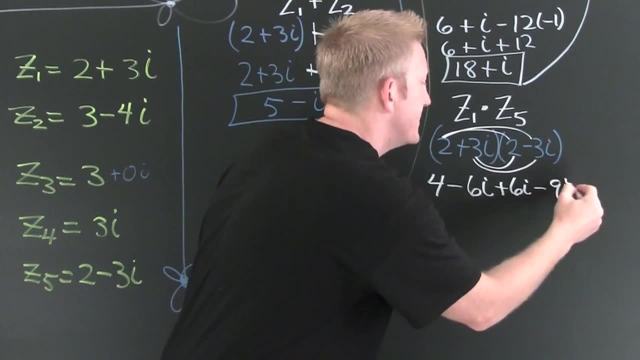 inner plus 6 and they finally laugh: that's minus. wait for it. nine eyes square. okay, they've had something go and they will go give me a very similar result in the pad. so that's the two plus zero minus 9. so time in our set of 3 five. 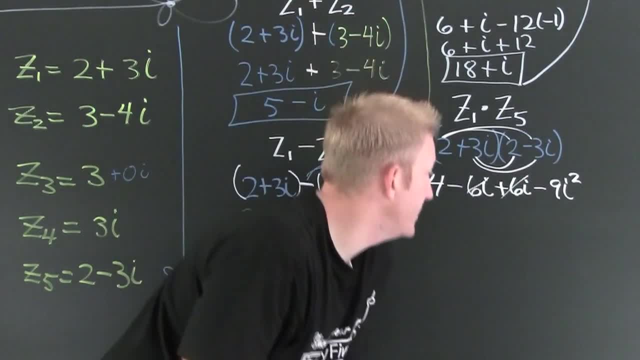 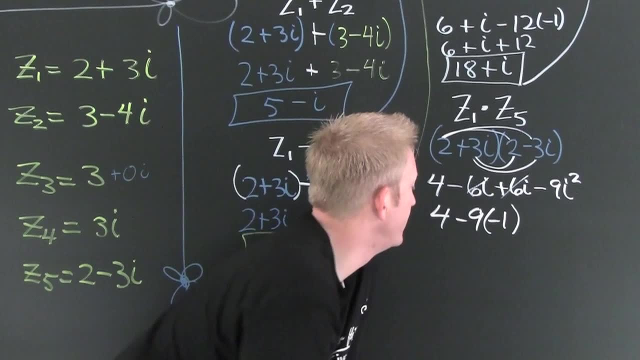 they like, top the systems and end this. the duration, marginalization, when niza was more than they're still additive inverses, even though they're imaginary. so then you have four minus nine times a minus one, fun, mm-hmm. so then this is four plus nine, which gets you 13. yes, 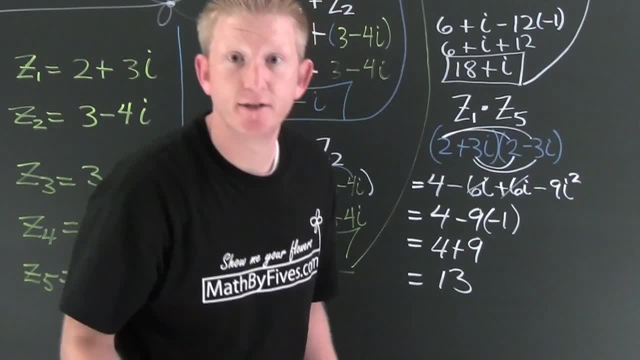 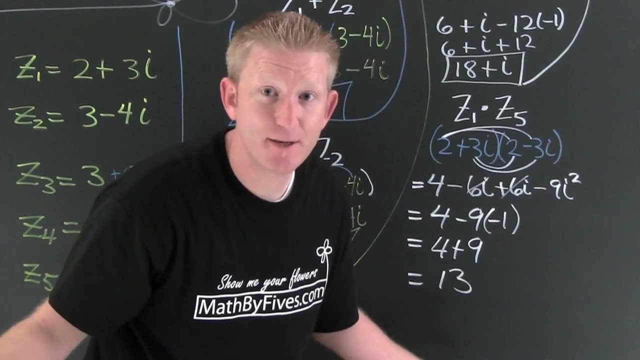 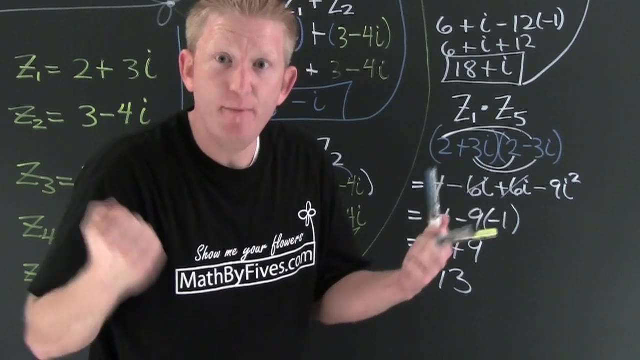 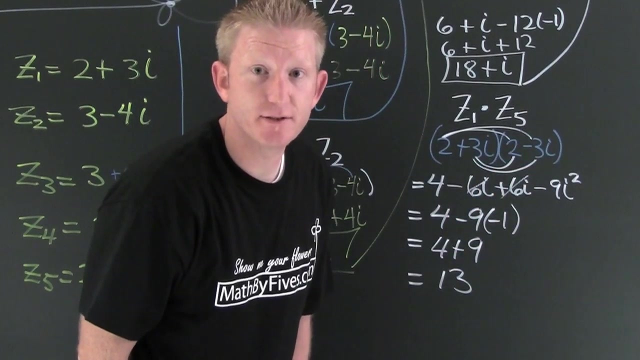 so what just happened there? I dropped my marker, no other than that. um, I took two complex numbers with imaginary parts, and I was able to get rid of the imaginary part. uh-huh, this is screaming difference of squares. uh-huh, something plus something, something minus something. so every single time it's this: 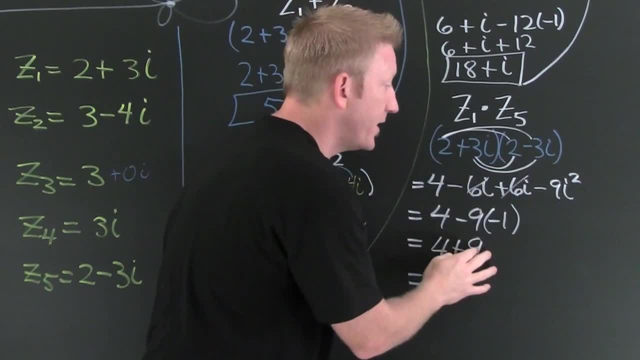 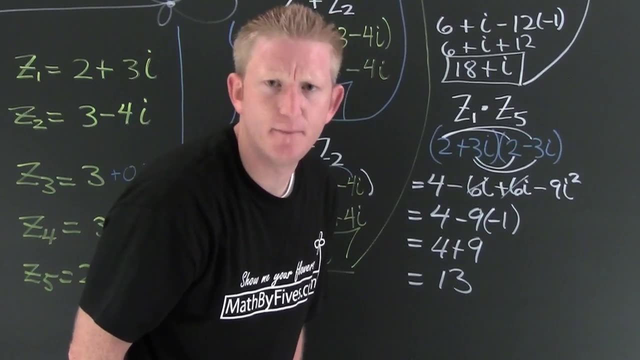 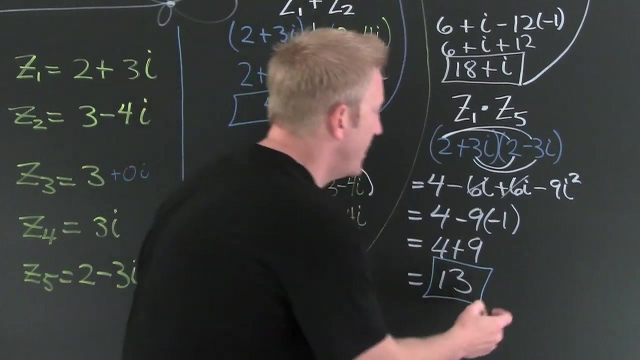 one squared minus this one squared, I'll be it. when I square the imaginary part, I'm gonna get a real part negative. some would even say that this is the sum of squares. oh boy, sure that was a cheap trick and I want to use this cheap trick on this division up here. 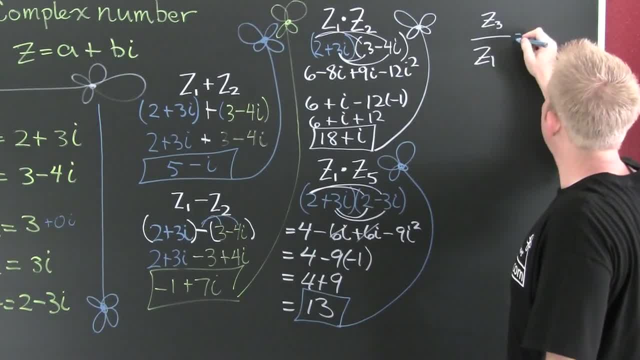 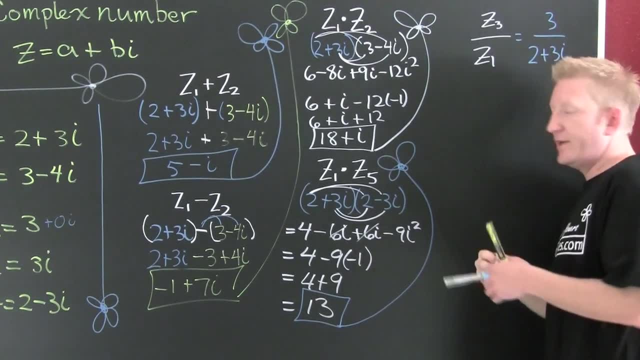 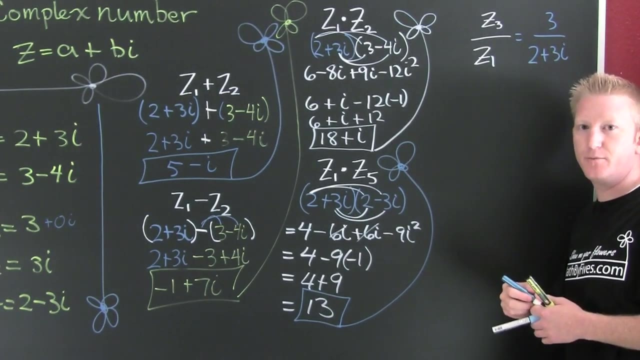 okay, so here's e3. it gonna be three, uh-huh, divided by two plus three. I now in my quest for division. I don't want that I in the denominator. so I need to do some something. I want to get rid of the imaginary part. you remember back when we 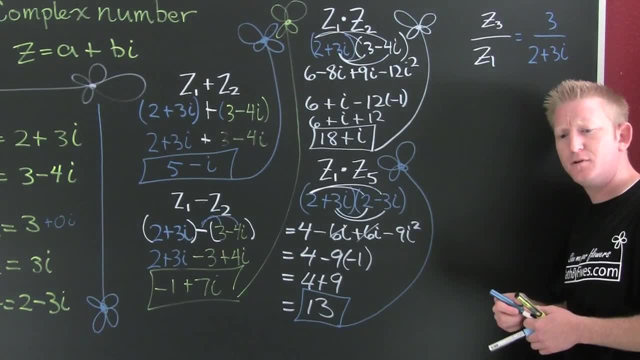 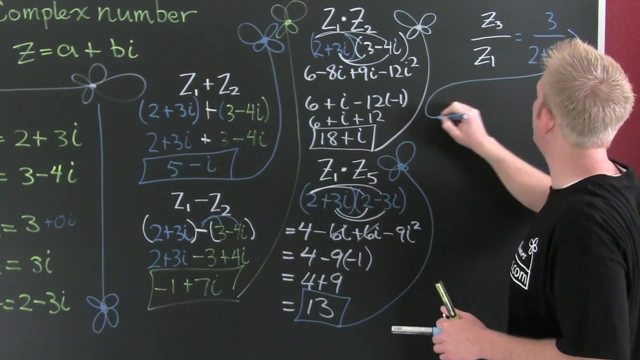 were rationalizing roots, when we had a root in the bottom and you had two terms. you multiply it by the conjugate. yes, and here we're gonna multiply by the complex conjugate. okay, I'm gonna bring this right on down here. I'm gonna have three. 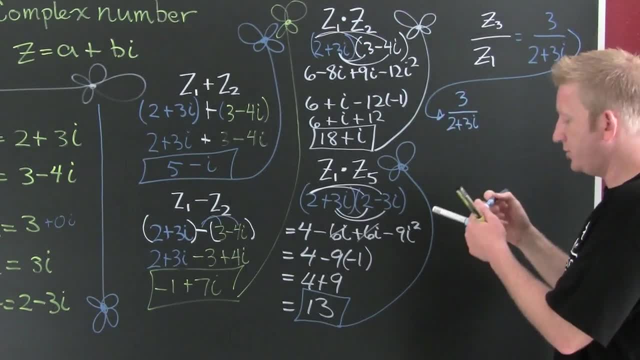 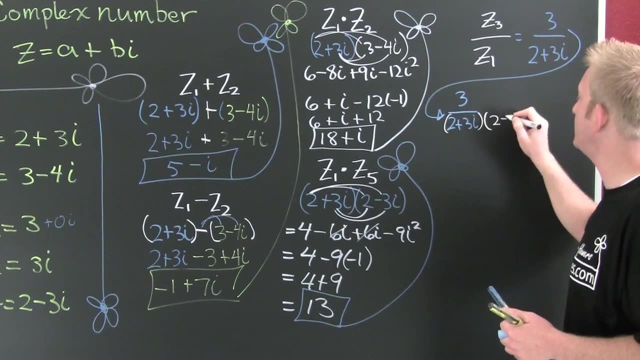 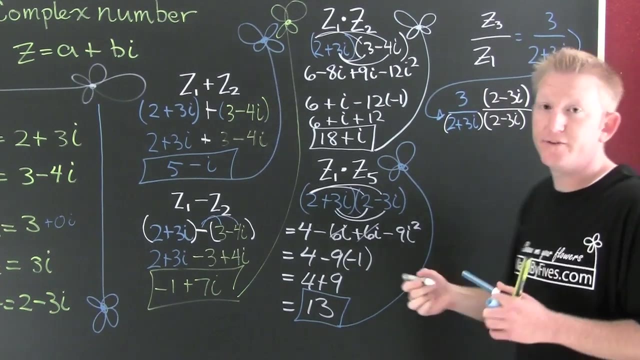 divided by two plus three: I okay, so I need to multiply top and bottom. okay, so I need to multiply top and bottom by the complex conjugate, the conjugate of two plus three, I is two minus three. I okay, I'm two minus three, I yeah. what are we going for? we're going for the 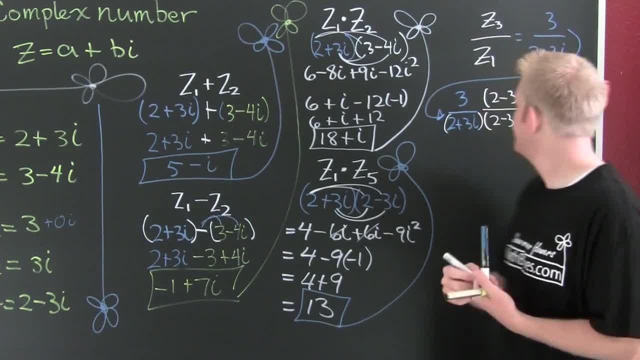 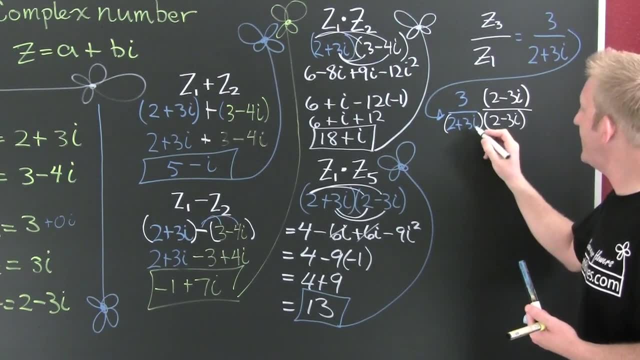 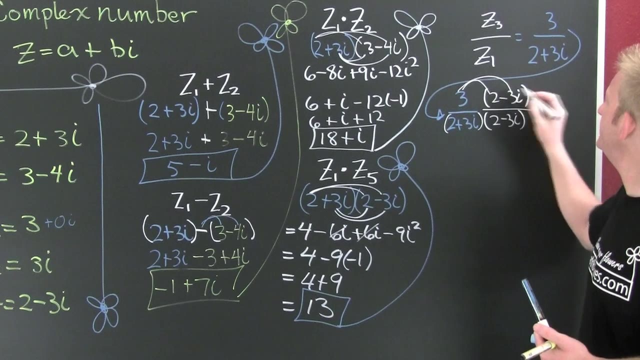 difference of squares and, in fact, this will turn out to be the sum of squares. yeah, okay, sure, now that I got that, alrighty. then I found in my last example this is gonna be 13. that was set up well, so then, up here to be, this is gonna be the sum of squares there. I'm gonna multiply this by two. 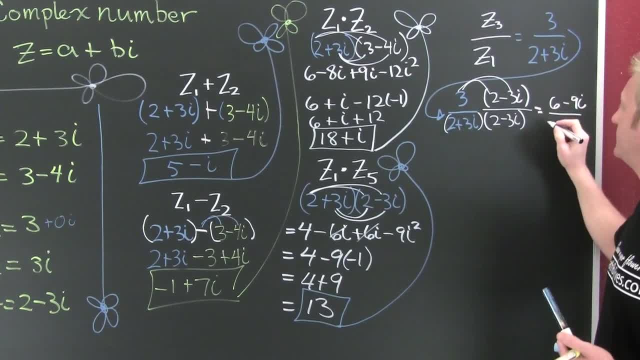 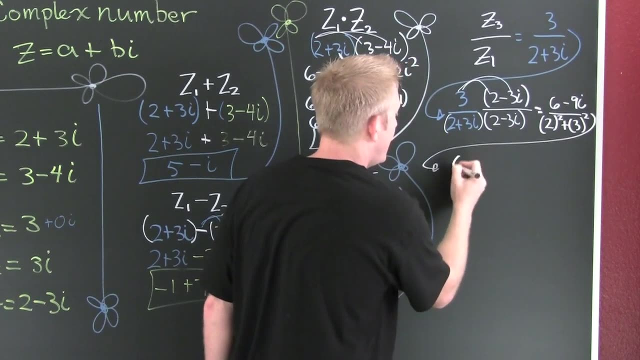 six minus nine I divided by this: one squared, two squared plus three squared. there I'm using the whole aforementioned sum of squares. so then I have six minus nine. I divided by- wait for it, wait for it- four, okay, plus nine. I divided by 2 squared plus. 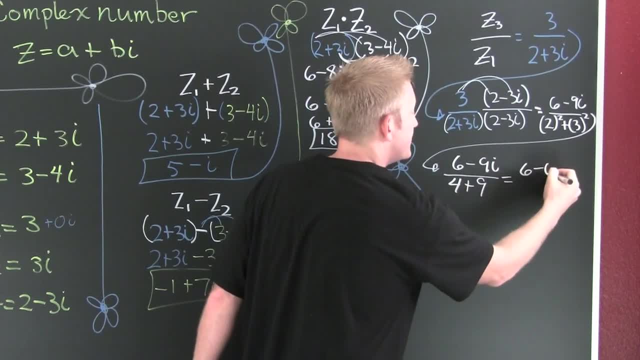 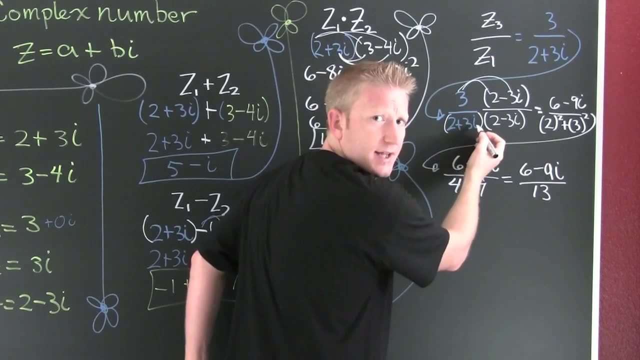 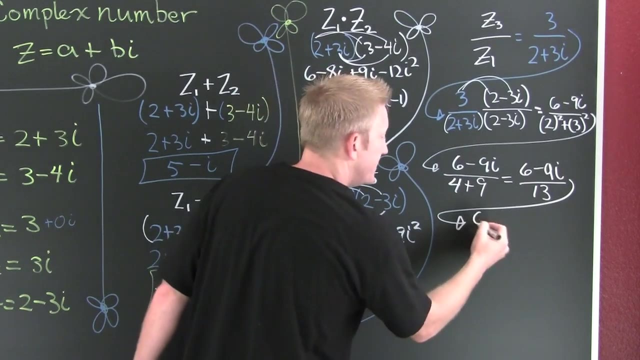 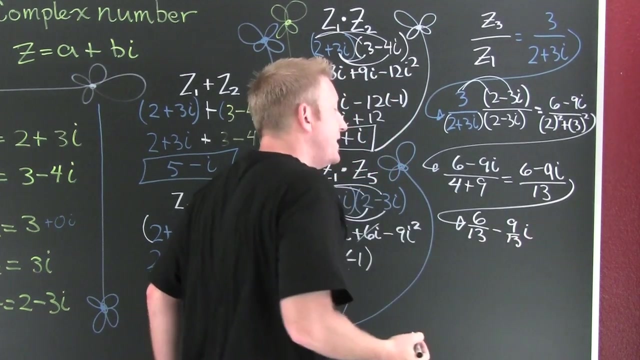 nine, yes, so then this is six minus nine i divided by 13.. if you're wondering how i got that, go ahead, foil that out, see if it works. now i'm not done there, because the complex number is written in a plus b i form. this is going to be 6: 13 minus 9, 13 i, and yeah, i want to write it like that. 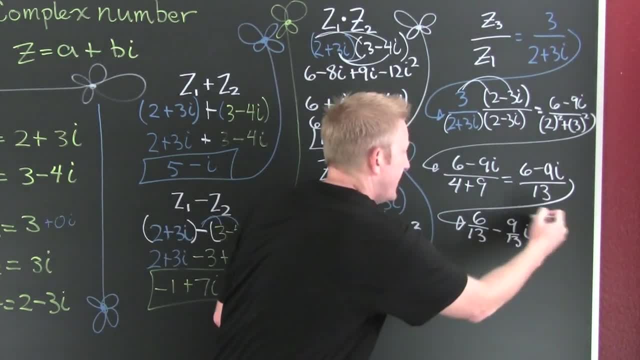 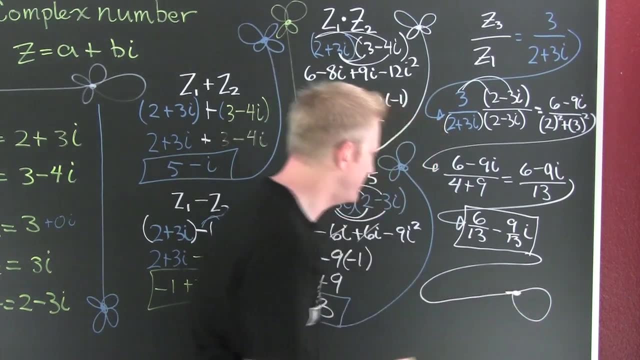 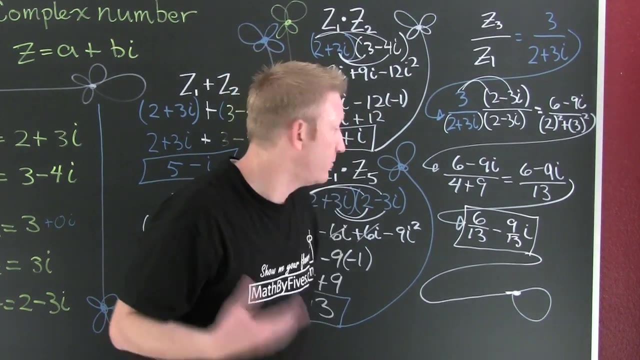 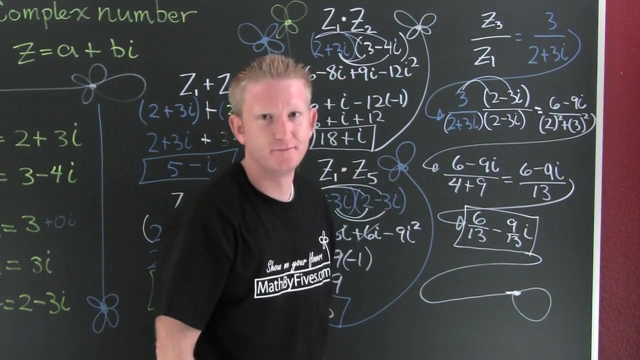 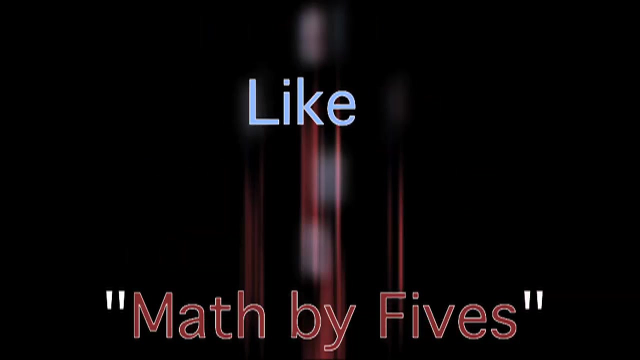 where i separate the reels and the imaginary parts, and then a box. hey, that's not a flower, what is that? it's a dog. remember back when you were at the county fair and stuff like that, sure, and you have those imaginary dogs, it's imaginary you.